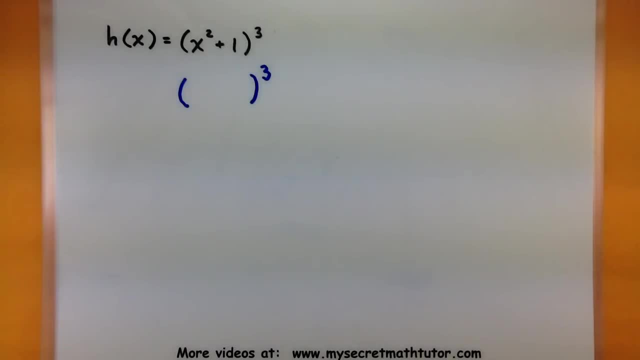 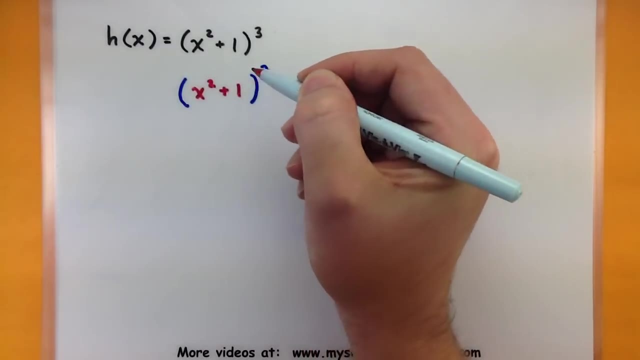 So I would really consider the The cubing part an outside function. It's taking something and cubing it. Inside of that we have an x squared plus one. So those are our two different layers that we're going to have to work with. 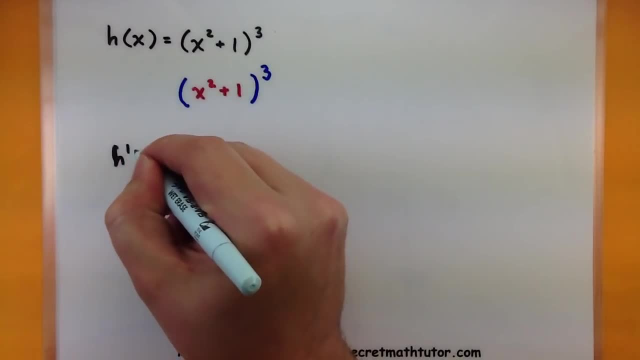 Let's see if we can actually do our derivative now. So I need the derivative of h, So we begin by taking the derivative of our outside function. So almost think of this: if I had an x cubed, what would it do? 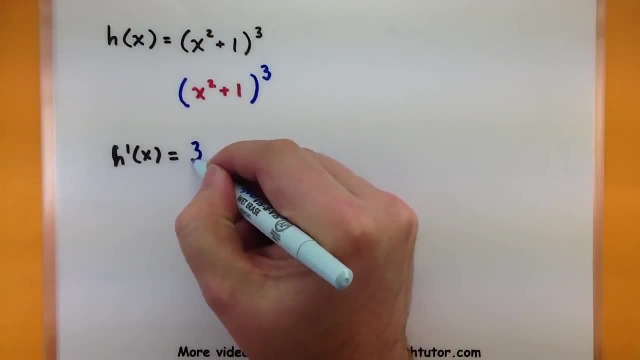 What would its derivative be? Well, you'd use the power rule on it, you'd bring down that three and you'd reduce that three by one. So you do the derivative of the outside just like that, and then you write the inside part. 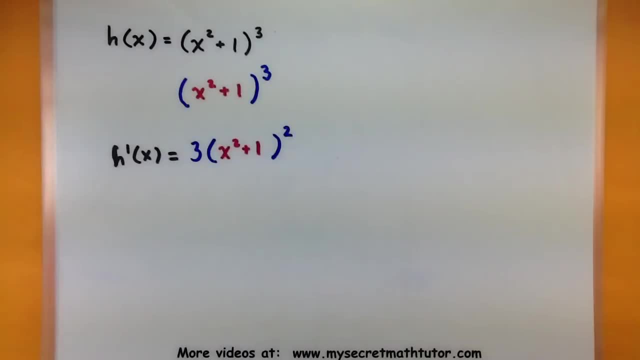 exactly the same, So this guy has not changed. Then you follow up by taking the derivative of the inside. So over here, when we multiply now, we'll actually take this guy's derivative. So multiply it by 2x, So that's the derivative of the outside. 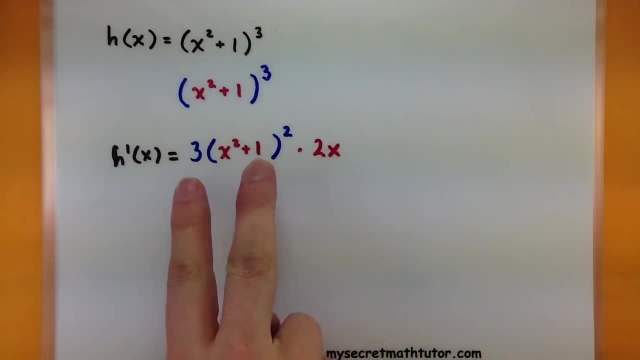 And then you do the derivative of the inside. Alright, so derivative of the outside: inside stays the same, multiplied by the derivative of the inside. Once you have all the pieces, let's go through and just clean it up just a little bit. 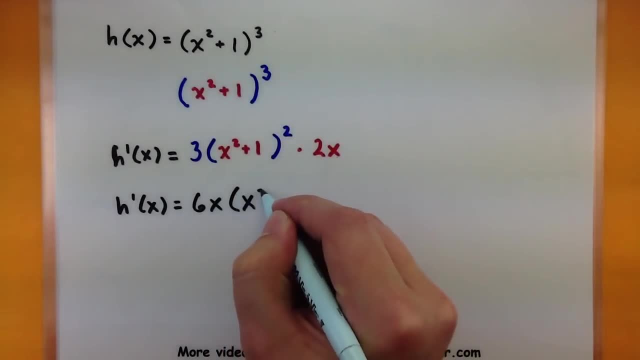 So 3 times 2 would be a 6x times an x squared plus 1, the whole thing squared. Now that's really tricky to watch. so let's look at two more examples. This one: we want to take the derivative of the square root of 5x minus 2.. 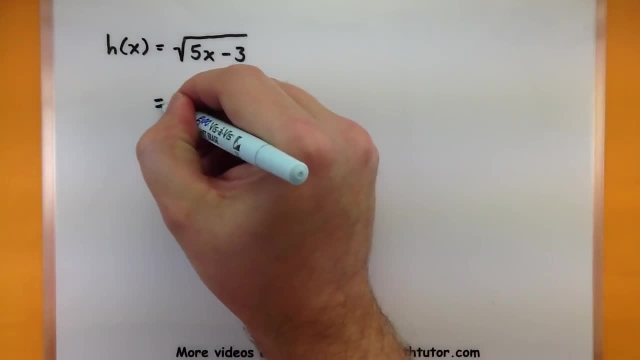 So, just like before, let's go ahead and highlight what the outside function is and what the inside function is. So we're taking the square root. that's really like our outside, and on the inside I have this: 5x minus 3.. 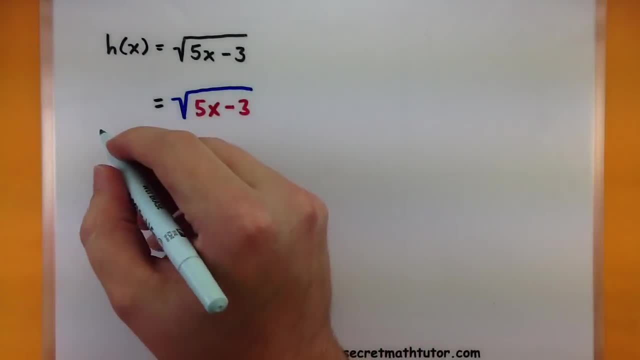 Okay, so what do we do when we need to find its derivative? Well, we'll start by finding the derivative of that square root, and one thing that will make that process easier is think of that square root as raising to the 1 half power. 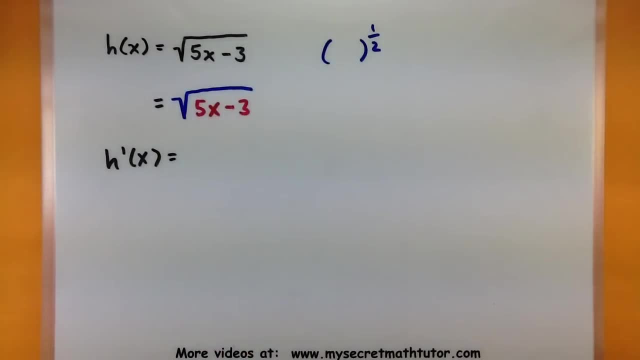 So what do we do when we need to take its derivative? We'll begin by bringing its power down out front, so 1 half, and then reducing its power by 1. So that will take care of the derivative of the outside. Straight into that we'll keep our inside function unchanged and then we'll multiply. 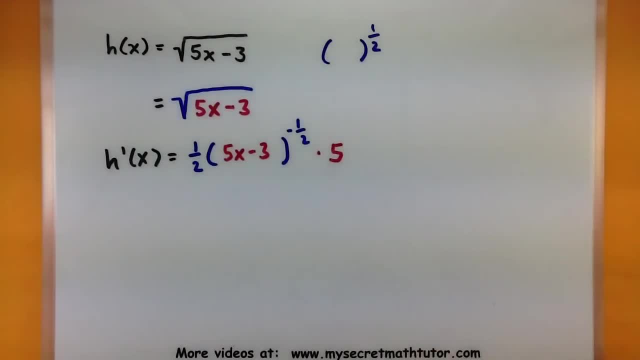 by its derivative 5.. Alright, now let's go ahead and clean this up. Let's see what do we got? I got 5 times 1 half, so I guess my 2 will end up on the bottom along with my square. 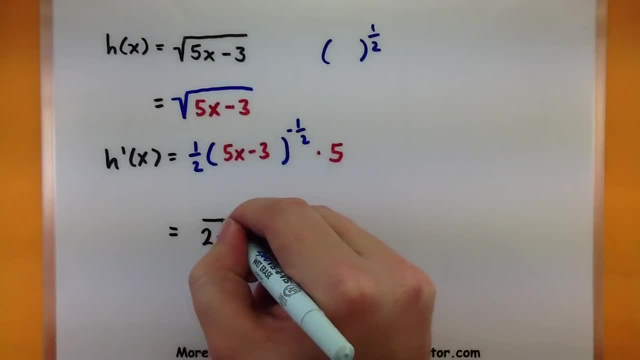 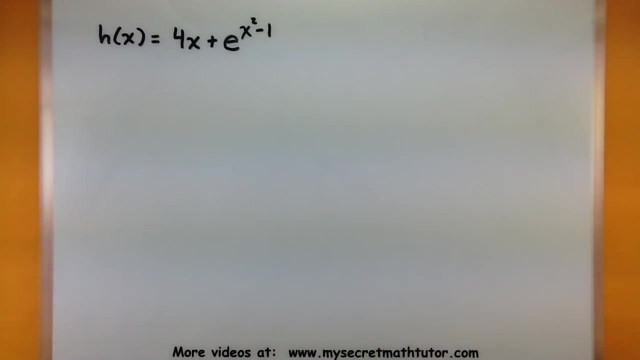 root, And the only thing left on top is actually just my 5.. So this would represent our derivative. Okay, let's do one more of these things, and this one's kind of a tricky one to recognize the inside or the outside. 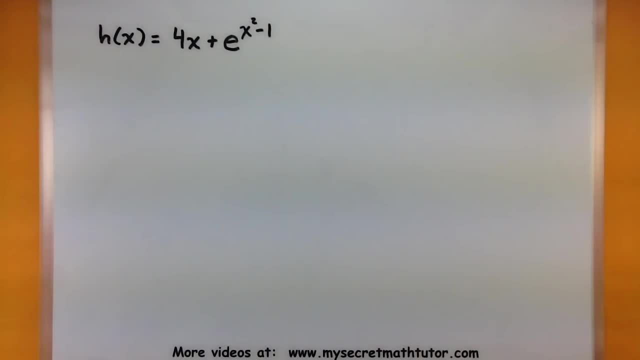 We want to find What is the derivative of 4x plus e to the x squared minus 1? Okay, and when you first look at this, you're like, wait a minute, aren't we really just adding functions? And that's true. 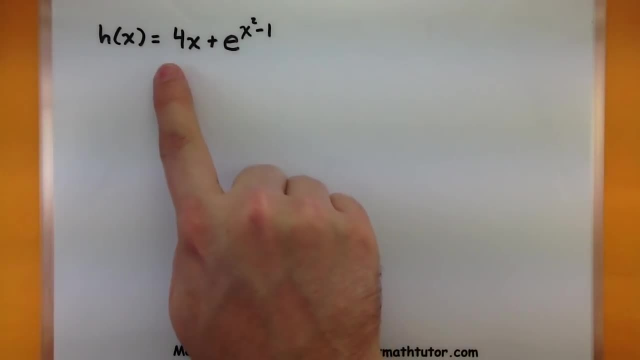 We will go ahead and use, like the sum rule for derivatives and look at the derivative of each of the pieces. It's this part right here where we will really need that chain rule, because we have a little function on the inside, that's the x squared minus 1, inside of our e to the x function. 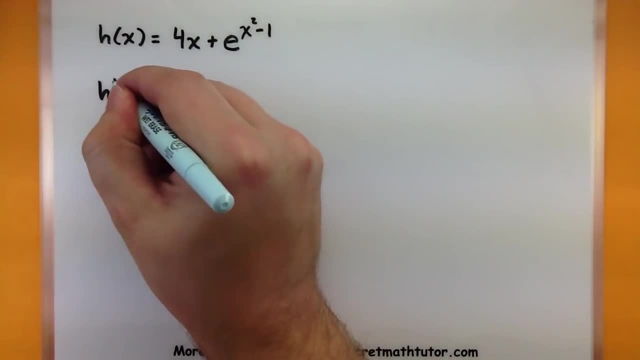 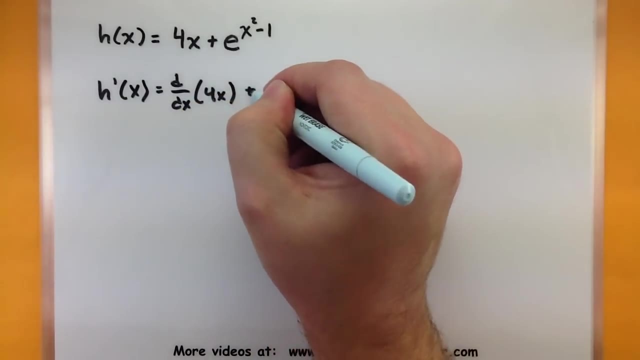 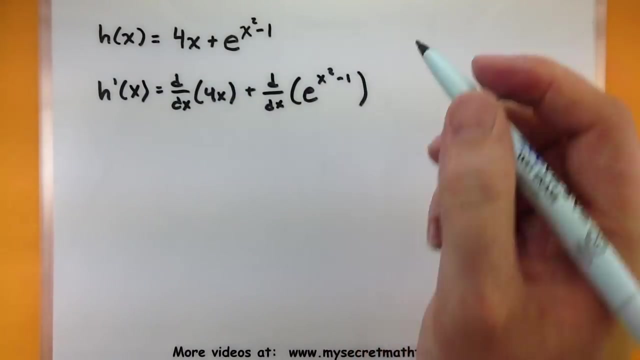 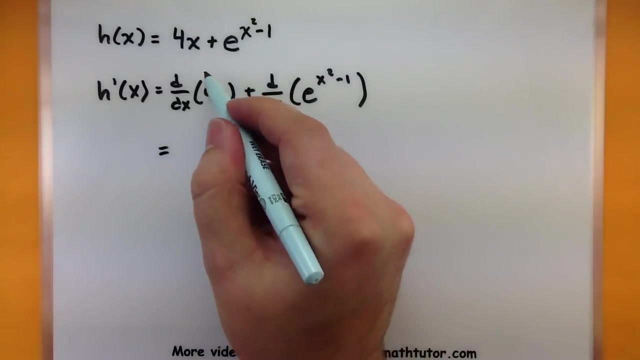 Alright, so let's get started. I'll say that the derivative of this function Equals the derivative of just 4x, plus the derivative of e to the x squared minus 1.. Okay, so we can take the derivative of 4x. think of moving the 4 out front and taking 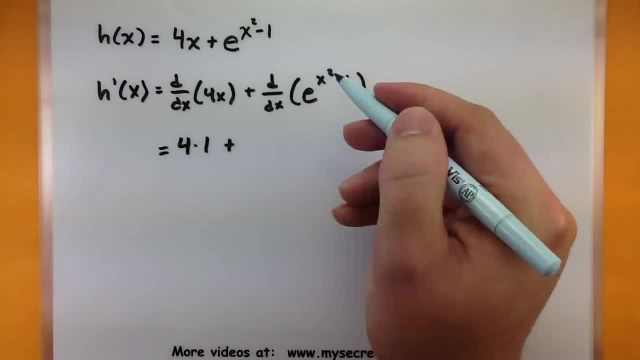 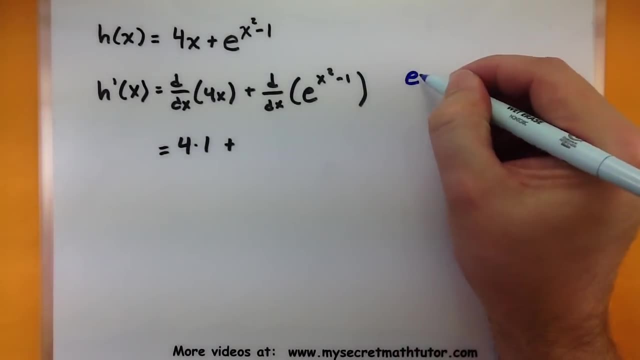 the derivative of just x, 1.. And now we've got to worry about this. Okay so, Okay, Okay. So what's going on here? Think of e to the x as your outside, and think of your x squared minus 1 as the inside. 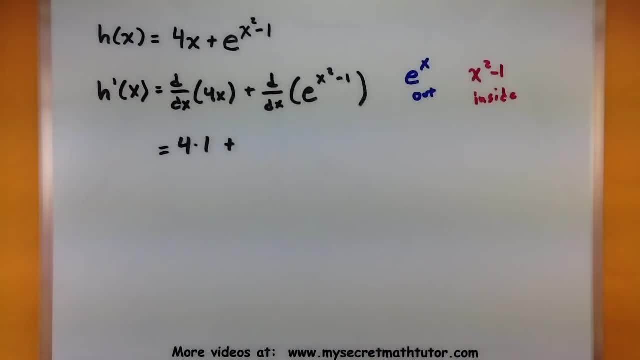 Alright, so remember, start off with the derivative of the outside. So what's the derivative of e to the x? Well, it's e to the x. But what do we put in the inside? Well, we put the function just as it is, unchanged.